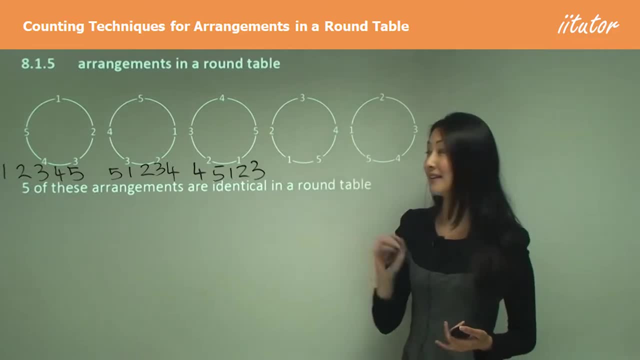 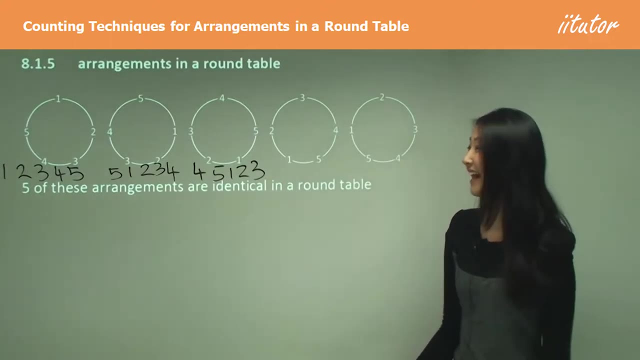 exactly the same. If there's five people around a table, there will actually be five of these arrangements. that's going to be identical. Yeah, and if there's eight people around a table, there'll be eight of these arrangements. that's identical and that holds true for no matter how. 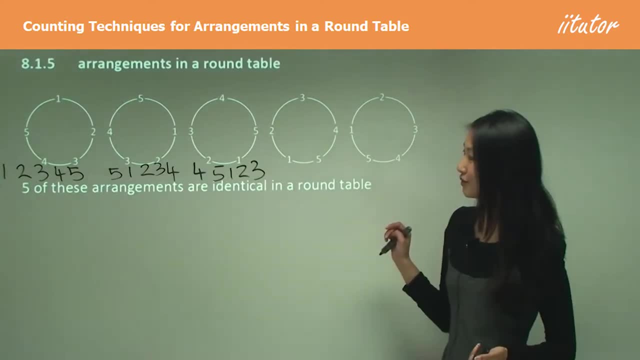 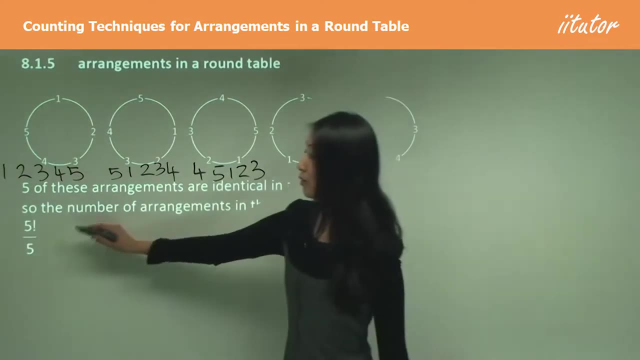 many people are around a table. So if you have five people around a table, you get four arrangements. number of people arrange in a circle. If that's true, then how do we work out how many arrangements there are? Well then we have 5 factorial. so if it was just in a 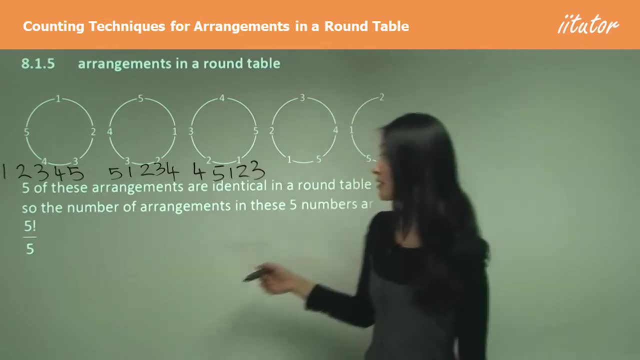 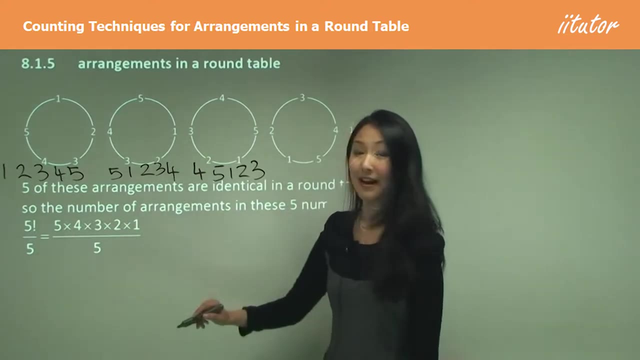 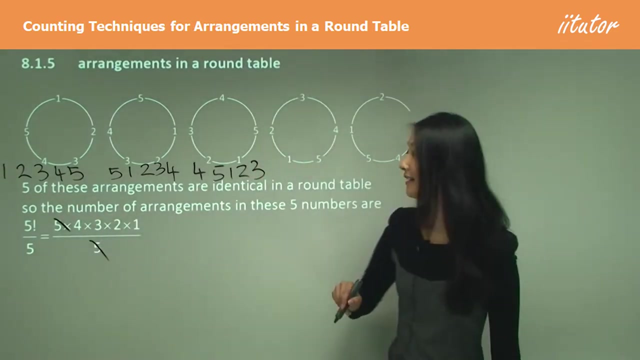 straight line, but divided by 5, so just dividing it by the number, arrangements that are identical. yeah, Now we can actually write 5 factorial as 5 times 4 times 3 times 2 times 1, cancel the 5s and this is the same as 4 factorial. 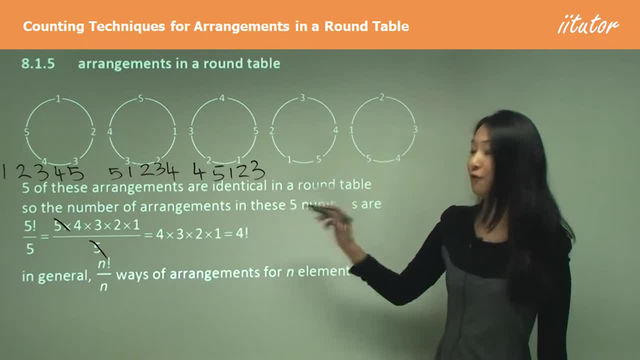 So for the answer here, it's just going to be 4 factorial Now from this, because I said it doesn't matter if you have 5 people in a table or 10 people in a table, it always works. so therefore we can come up with like a general rule and 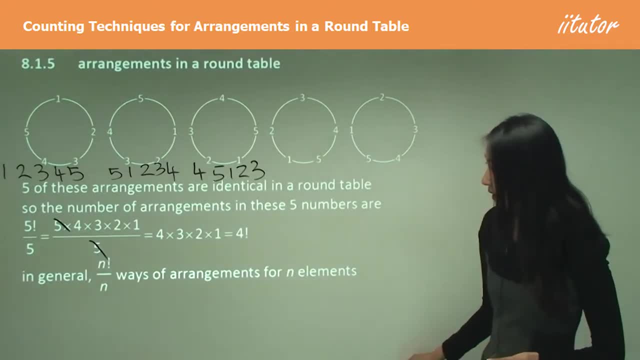 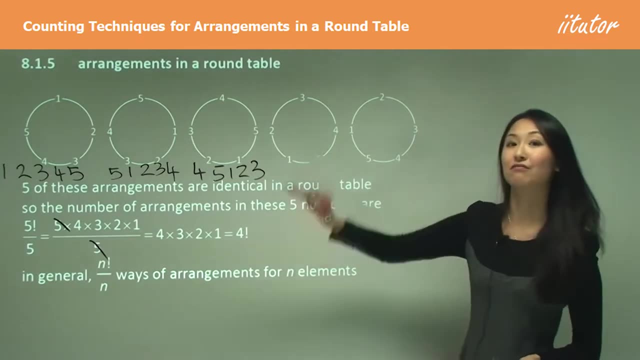 the general rule that we've came up with is that n factorial divided by n ways is equal to 4 factorial. So that's the general rule that we've come up with, and the general rule that we've come up with is arrangements for n elements around a. 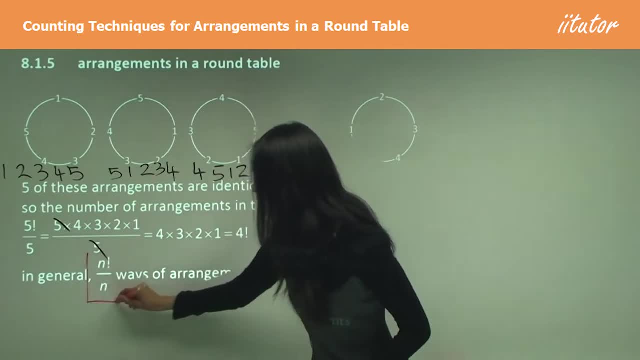 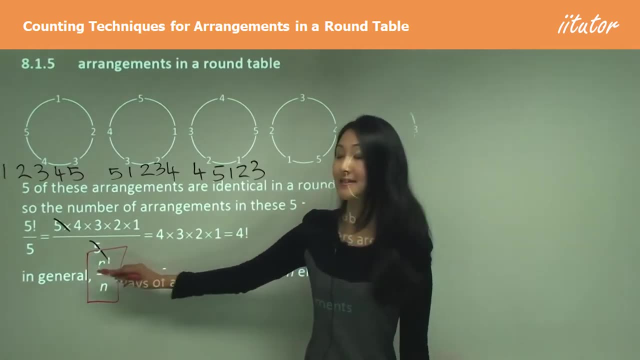 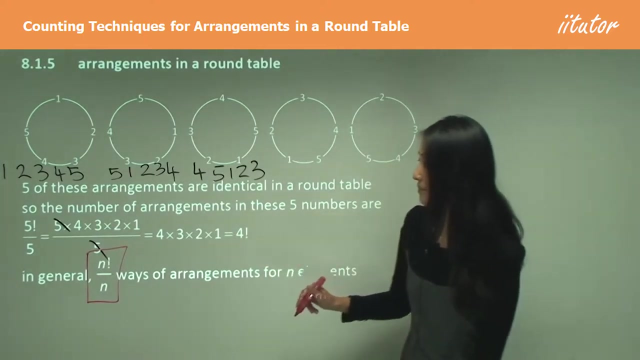 circle. So that's just your algebraic way of saying that when you have people or things arranged in a circle, you have that number of objects, factorial, divided by the same number, because that's the number of repeats Sometimes. so let's consider our n factorial divided by n. so in that case sometimes you'll see your. 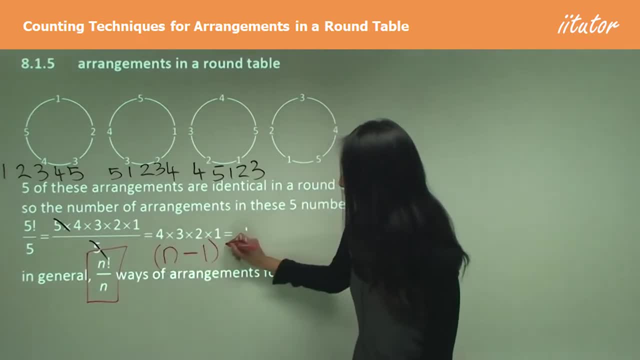 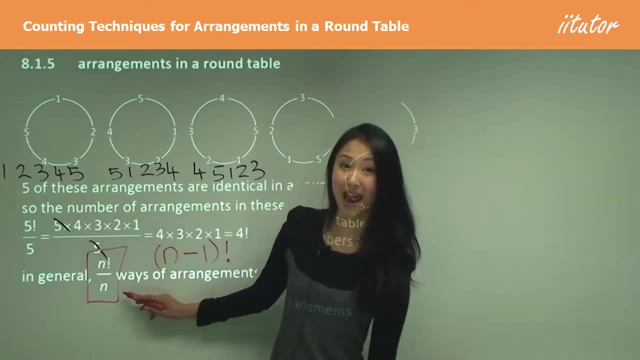 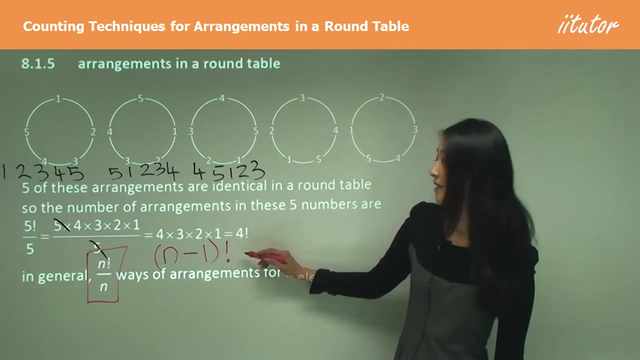 teachers write n minus 1 factorial for circles, and that's because you can see, when we have 5 factorial divided by 5, so n factorial divided by n, When you solve it like this it actually becomes 4 factorial, so n minus 1 factorial. so if you say this, just know that it's derived. 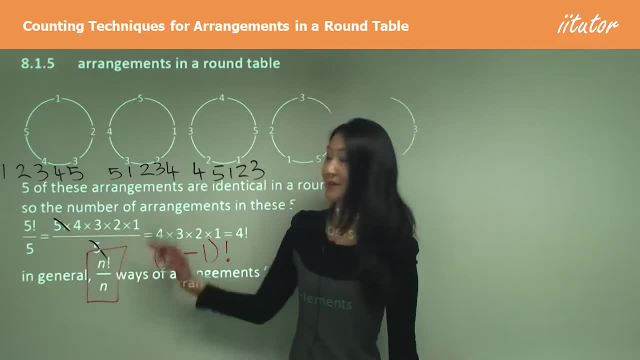 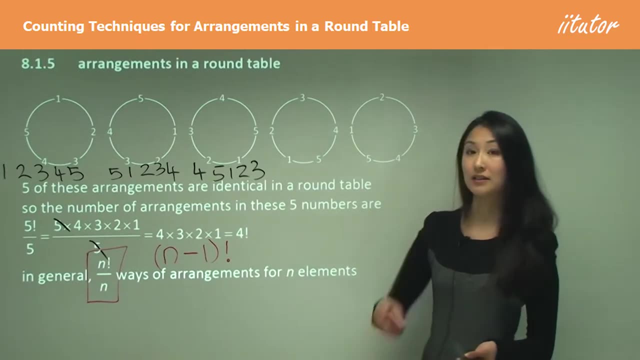 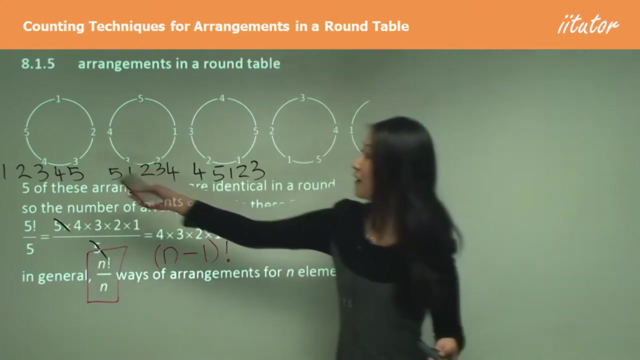 from this general equation here. okay, Because this is the proper way to explain why this is. yeah, So just understand that when we're arranging people or things, it's intrinsically different from a straight line, because there's gonna be repeats. Yes, things that are different in a straight line. 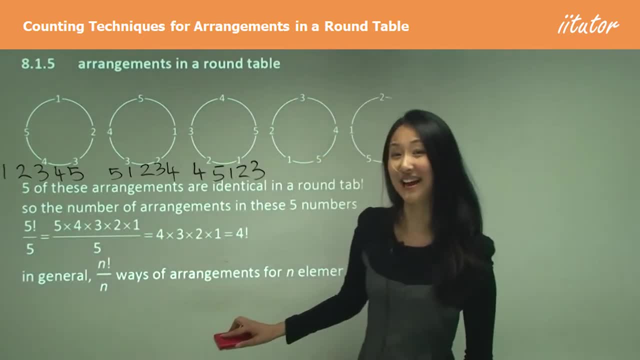 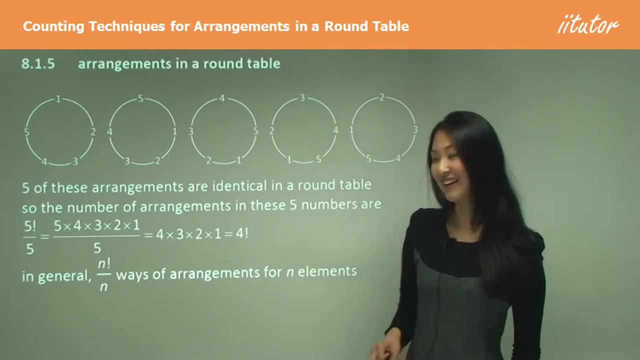 when you join them together to be a circle, they're gonna be exactly the same, And if there's five people, there'll be five arrangements that are exactly the same. so we divide by five. okay, All right now, as always, with our factorial questions. 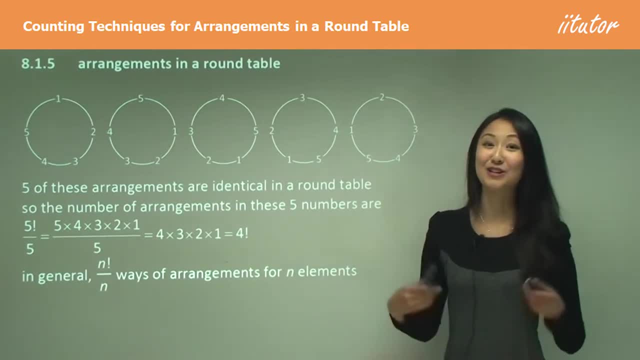 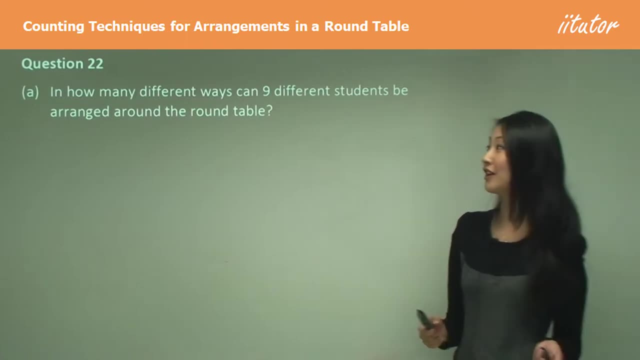 and permutations and combinations. best way to learn them is by doing questions. So let's have a look at question 22 here. So here we have nine different students arranged around a round table. So let's just say for your formal, And how many different ways? 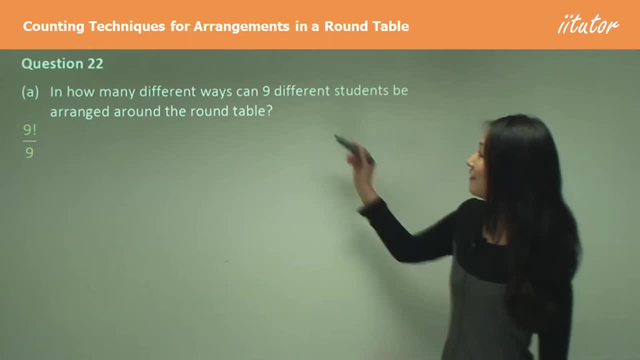 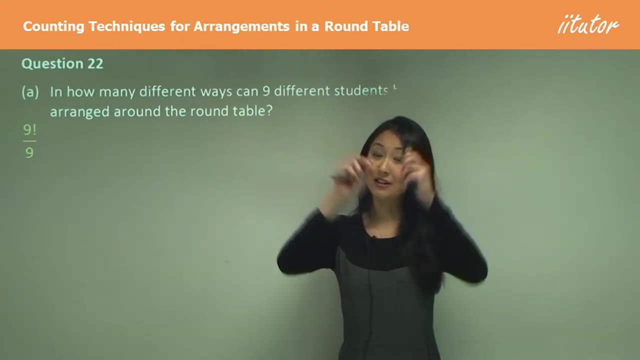 can they be arranged around a table. So consider: there'll be nine students, So it'll be nine factorial if they were standing in a line together. But because we're putting it together in a circle, there's gonna be nine repeats, so nine identical tables. 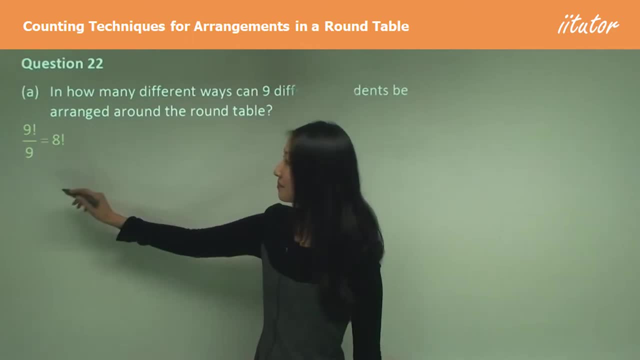 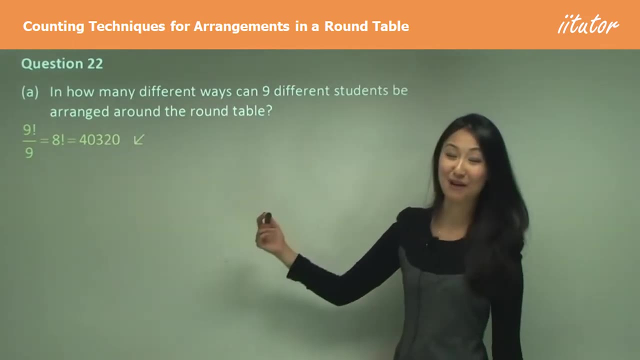 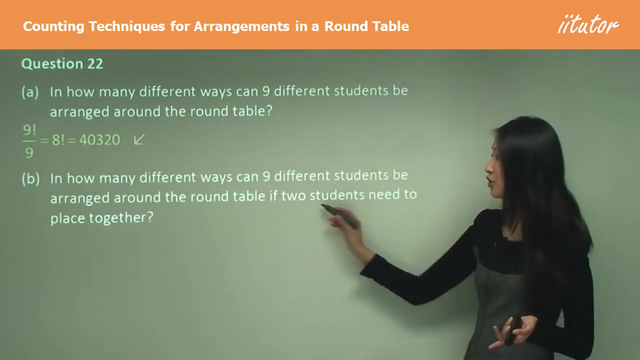 So that's why we divide it by nine here, which is actually the same as eight. factorial, which is 40,320 way arranging people around a round table, which is actually quite a lot of ways when you think about it. What about if two students need to sit together? 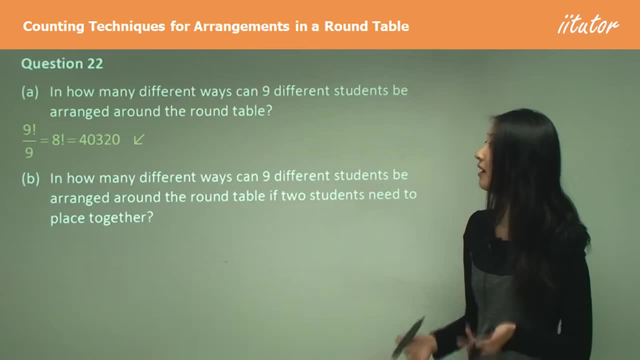 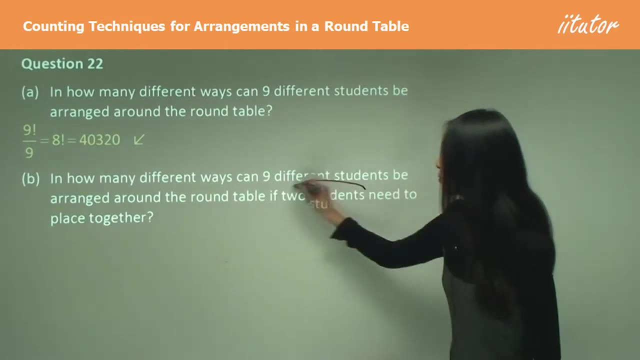 So let's say there's two people who are best friends and they want to sit together. How do we work that out? Well, how do we work out those before? If two people need to be together, exactly, We group them together. 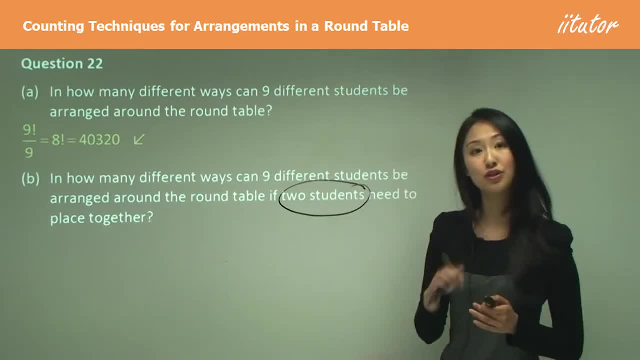 so we just group the two students together. If we group those two students together and we count them as one, instead of there being nine different student groups, essentially there's gonna be eight of them. yeah, because we're considering them as one. 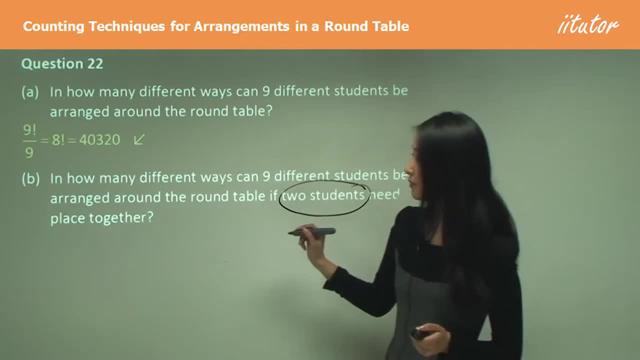 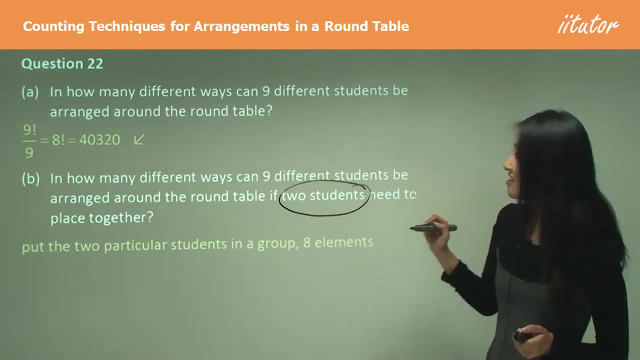 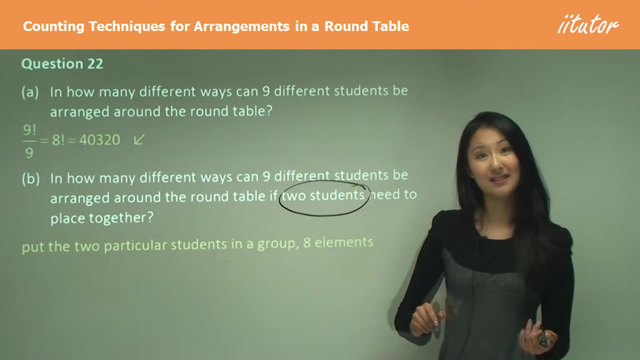 So that means I'm gonna have eight factorial. So put the two particular students in a group so there'll be eight elements, so eight factorial. But now they're in a circle so we're gonna have to divide by eight The number of identical elements. 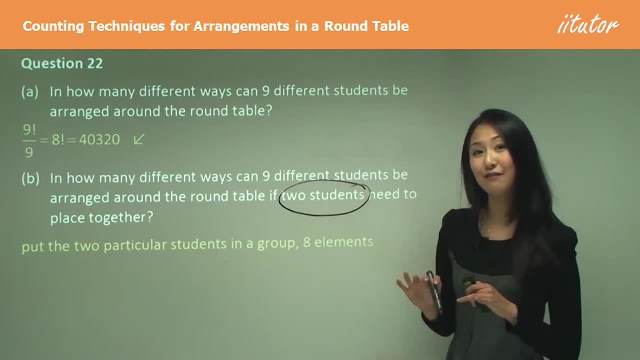 So there's eight groups, so we divide by eight. Now, be really careful not to divide by nine, because we're grouping those two students together. so there's only eight groups. So then that's why we have eight factorial divided by eight. 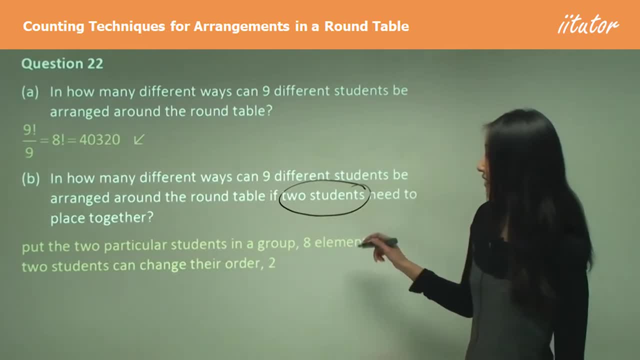 Just remember, when we group things together, unless it specifies one person is behind another or one person has to sit to the left of another, those two students say A and B can be A B or B A, So they can change. 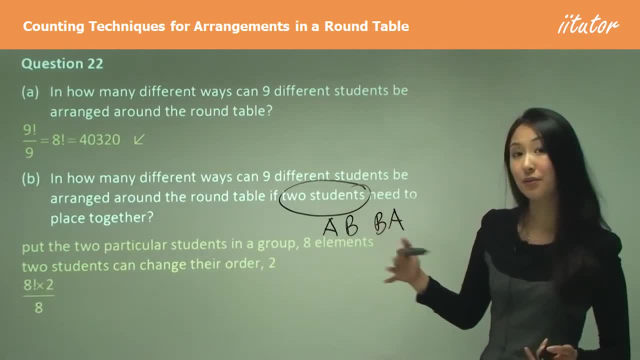 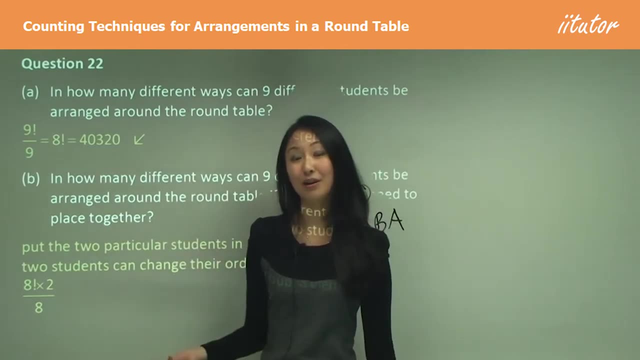 so that's why we can multiply it by two factorial. So what we have here is eight, factorial because we grouped them, divided by eight because of the circle. so there's eight repeats multiplied by two. factorial because those two people that are grouped together 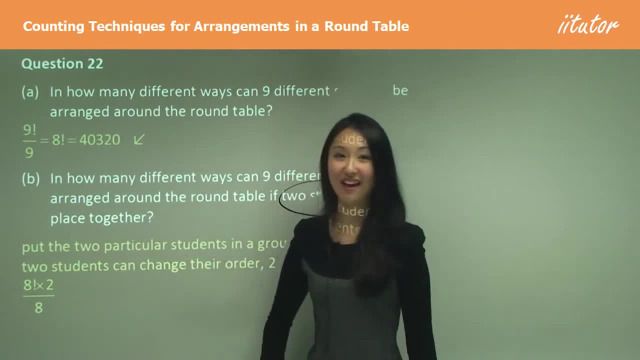 can change positions, And that's how we get that solution there, And you can just put that in your calculator. So that just becomes seven factorial times two And that gives you 10,080 ways. all right, So if coming straight to that becomes confusing. 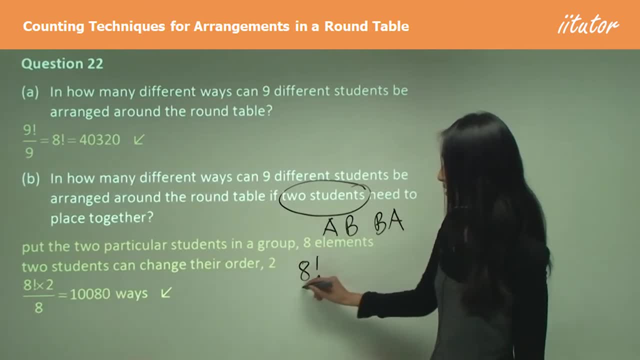 just start off with thinking it's eight factorial. Now it's a circle, so I divide it by eight. but because I group them together, I need to multiply by two. Just work through it slowly, through all the different elements, and you should be okay with that. 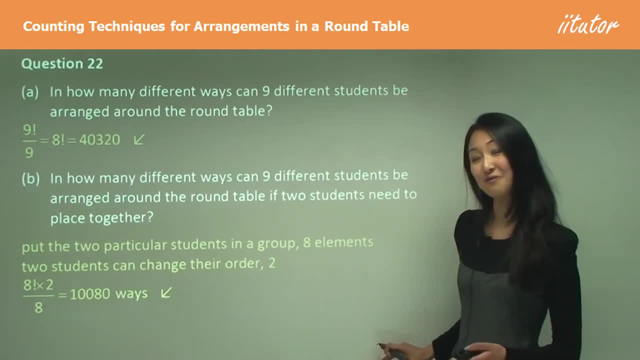 And always remember, if you're grouping people together, always consider the arrangements within that group. Now we come to the question, which is: can we divide by 10,080?? Can we divide by 10,080?? Can we divide by 10,080?? 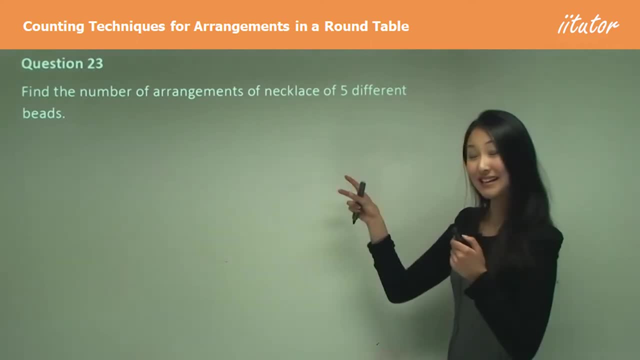 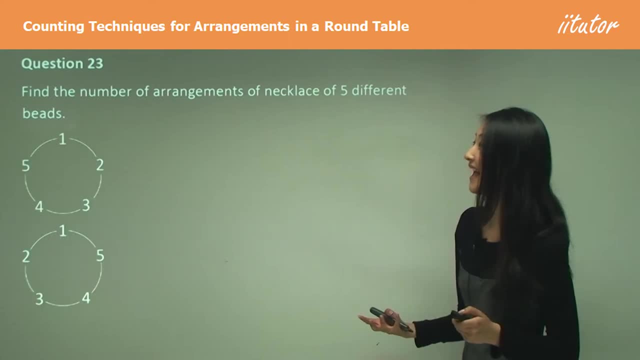 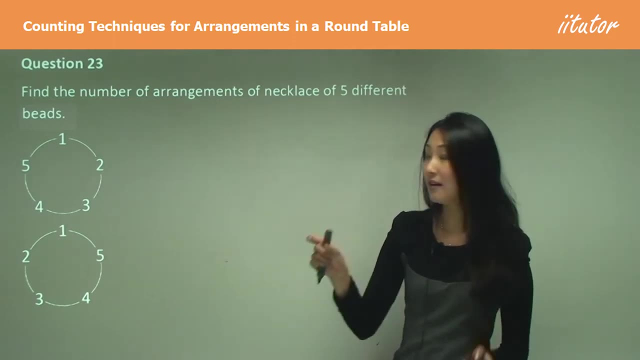 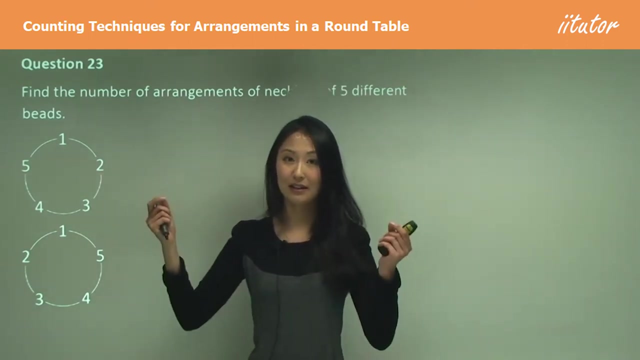 very special way of arranging themselves, and that's because, when you consider a necklace right- and let's just say they're beaded necklaces- yeah, so I have these five beads here. this necklace is exactly the same as that, because with a necklace, you can just flip it around. yeah, so wearing this necklace is exactly. 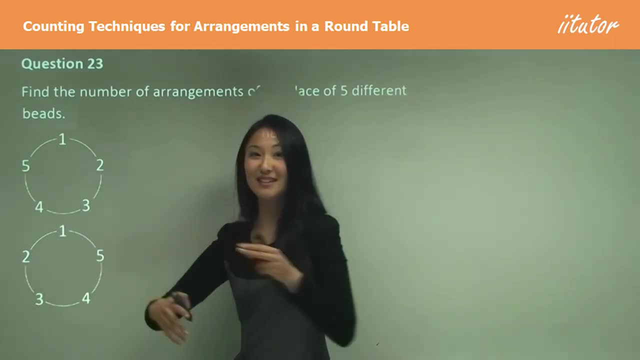 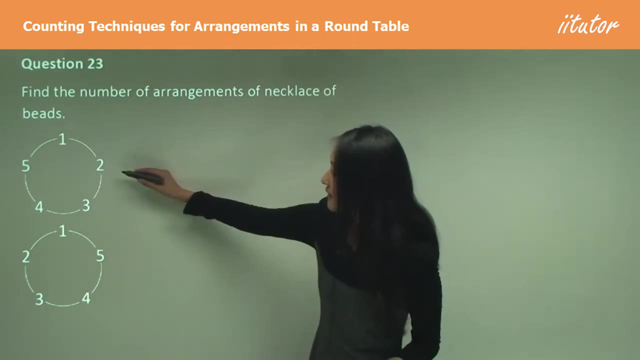 the same as that. that's just flipped around. okay, but this doesn't apply to people, because basically you can't flip a whole table around. yeah, you can't flip people around if you have this and then two is sitting on this side of one and two sitting on the other side. so that would be different for people, but only.